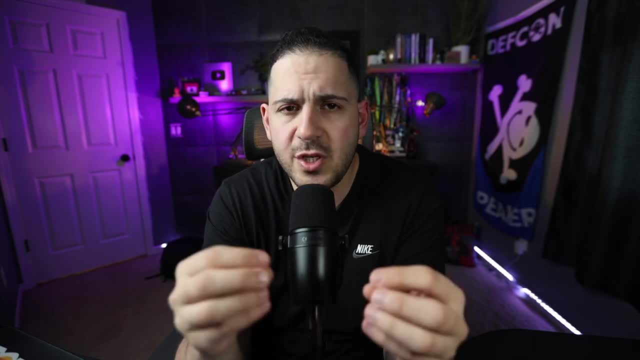 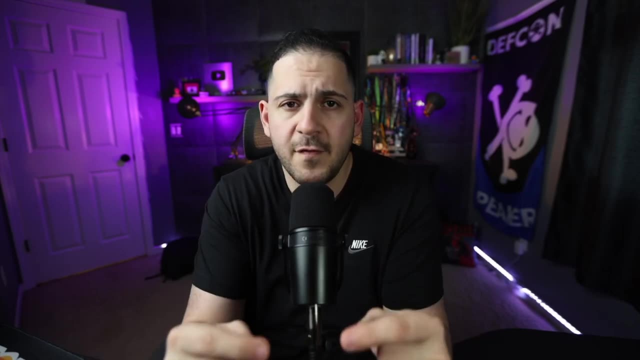 will show you in just a sec. In either case, it is allowing you to inject malicious javascript code within that website and you can kind of control the browser's behavior in the context of that specific target. So, for example, if you inject a cross-site scripting payload in a website like 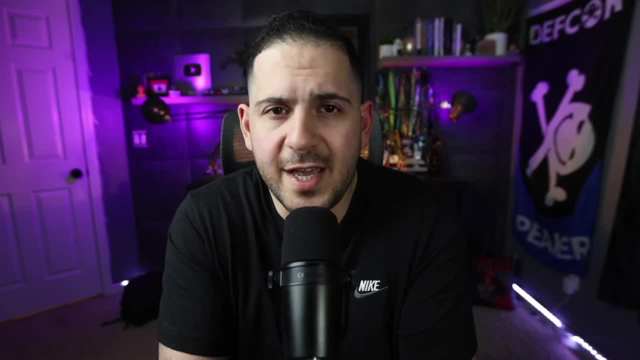 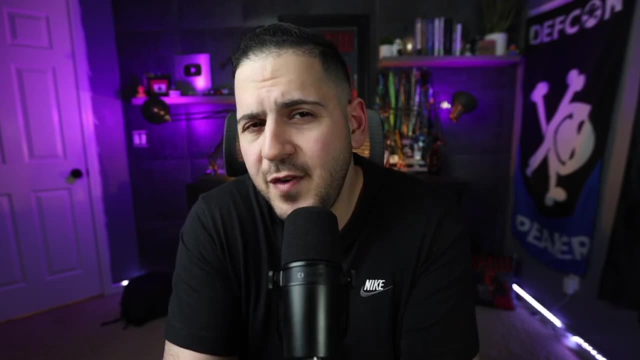 amazon. you can potentially take over their account. you can make them shop and buy whatever item you want them to, and that kind of stuff is what you can do. The account takeover- part of it could mean a lot of different things. sometimes you can hijack the entire cookie and you can log in as them. sometimes you can hijack a api key, for example, and log in as them, and there are other tricks that you can do, but in the general, the XSS thing at the root of it, it is all the same. it's just finding an html tag that you can inject, then escalating that to javascript. 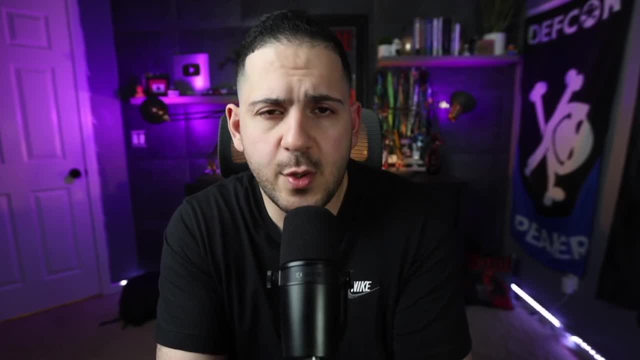 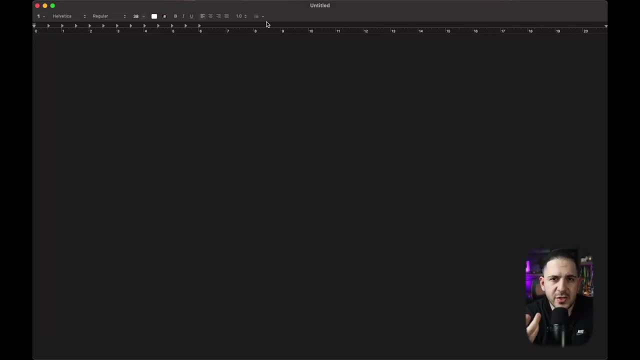 and then reporting that to a bug bounty program, a vdp, or even if you are on a pen test, you can report it as a finding on your pen test. Before we jump into our demo, let me explain how javascript in the context of XSS works. So, for example, when I say: I want you to look for html, 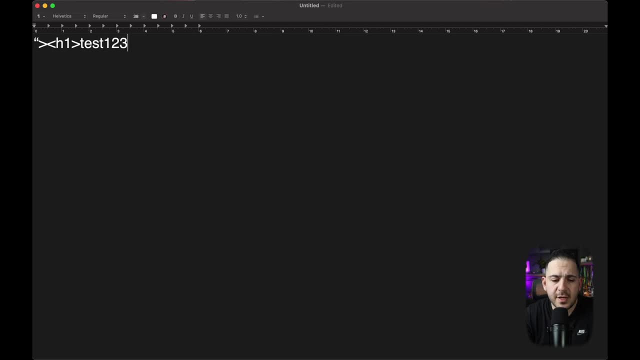 injection. first, all you have to do is do something similar to this which says: hey, I want to insert a h1 tag. it could be an underline, it could be a image, whatever you want to do, but I always start with a simple html payload that says: just test one, two, three. and then I'm going to show you how. 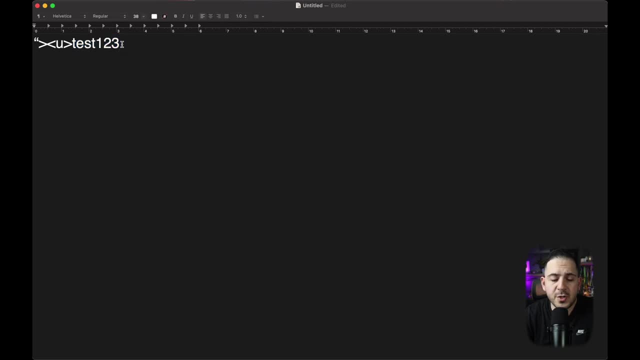 to look for that in the next step, but this is what I usually use. and then if that actually renders, and if it underlines and comes back with something like this, for example, on the page, then kind of know that hey, this reflects and it's also rendering that html and there's, there might be. 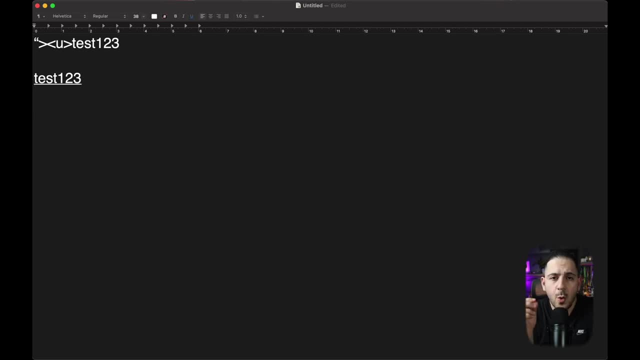 some sort of vulnerability here. so next, what you want to do is you want to introduce what is called an event handler, which is where you tell it on a specific event. you want it to call out a javascript function. so, for example, we can say, hey, I want you to do this same underline, but now I want you to 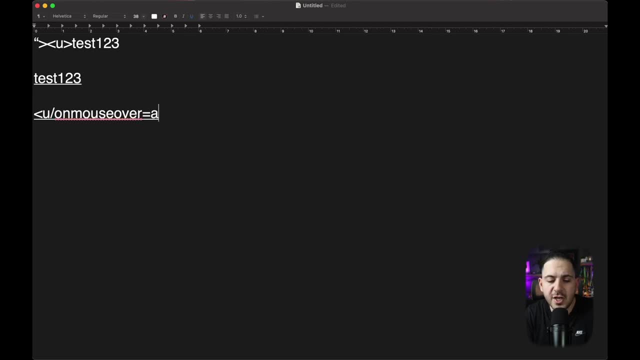 say on mouse over, I want you to call this function called alert and I want you to alert with the pop. so you say: test one, two, three, and what happens is when you pass this, the application is going to give us the same thing right here with the test one, two, three. but when you hover over it- because 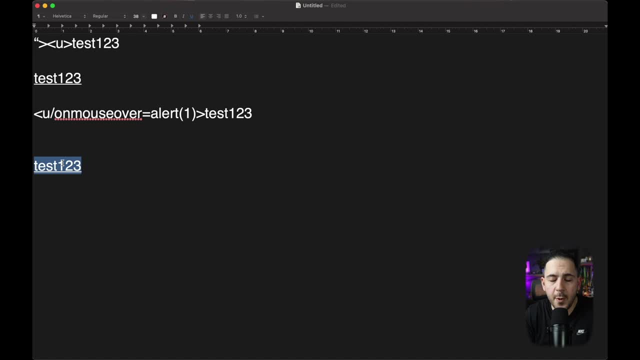 you said on mouse over alert one, it's going to pop up with an alert. so it's the same thing when you do a image source equals x and you say on error equals alert one. the reason why that works is because this x doesn't exist. there's going to be an error with that image and it's going to call. 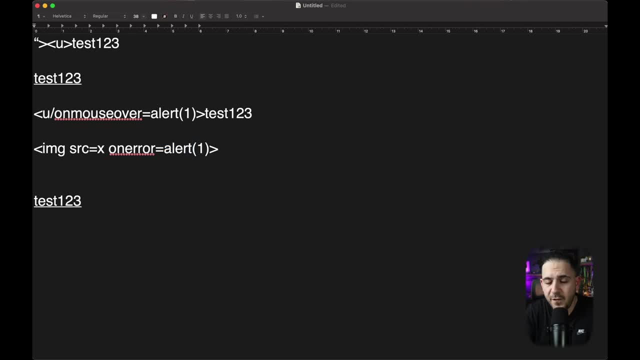 alert for that specific reason. so you can also do other functions. you can do something like: uh, confirm. for example, you can do import, if you want to import your own javascript code. so you can say: import my sitecom slash 1.js. or you can put them in quotation marks as well and you can put. 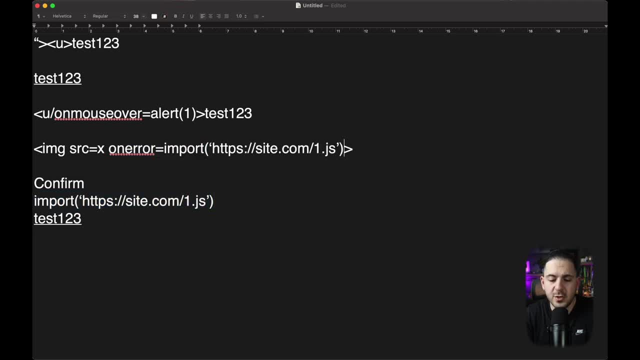 that on error right here. so every time there is an error it's going to call out to your javascript file and it's going to execute whatever is inside of it. so in onejs you can put something like alert one or, if you're more advanced, you can put your xss payload or your blind xss payload within. 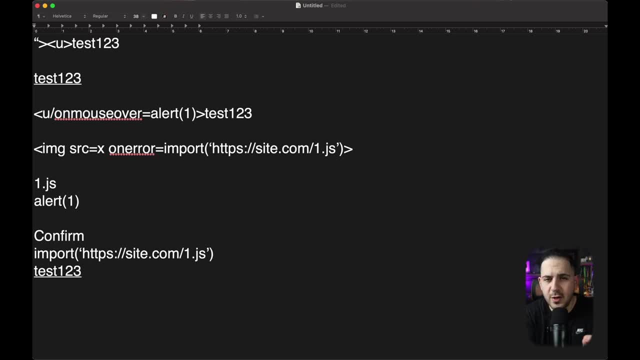 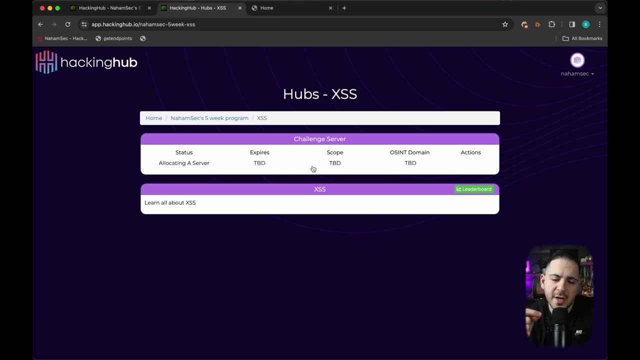 it and call it every time. so I want to make sure I cover that kind of understand how javascript works and why these event handlers work, before you jump into cross-site scripting itself. now let's jump into our example and, as always, you can follow along by going to hackinghubio. just look for my five-week program hub in there, go to xss and we're. 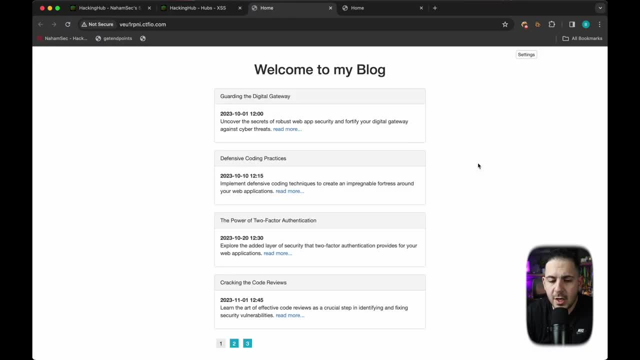 going to launch it. give it a sec. it's going to come back with a URL and you're going to click start. it's going to bring us to this website. you are going to need kaido more than likely. honestly, it doesn't matter what tool you use. you can use zap, you can use burp community or you can just do. 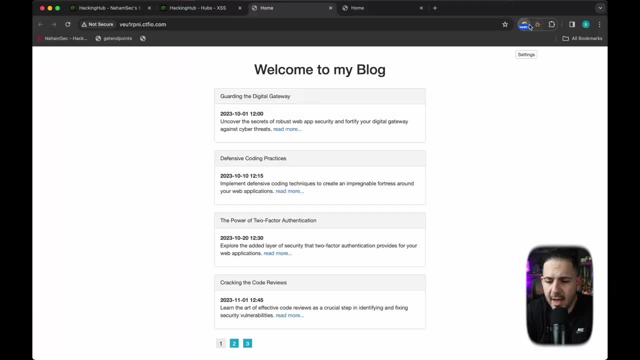 whatever kind of kaido I'm using is a free version. but here we are. we're going to activate our burp suite. it is already active and it's going to intercept it whenever we need it to. but the first thing we want to do is we kind of want to look around this website. I'm sure there's going to be. 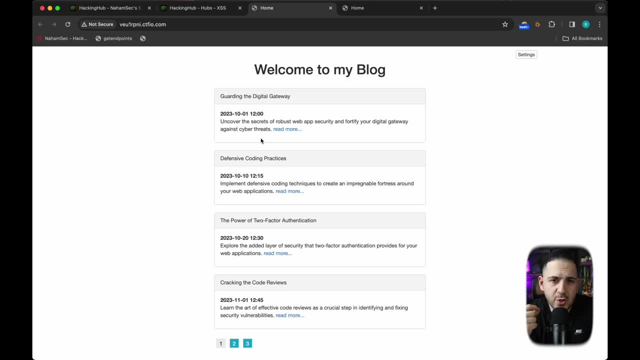 a lot of xss in this one, but I'm going to cover a few of them and show you how I look for them specifically. the number one thing you want to do, obviously, is you want to click on all these different URLs and see if it does anything and if it takes a different page and if that page 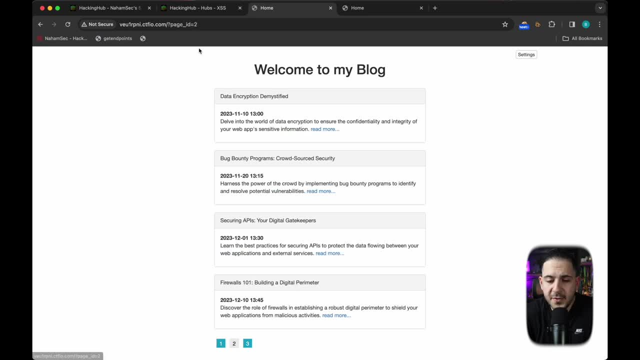 actually has any functionality. this one doesn't. this one is going to be going to the next page, which is going to add the page ID too, and usually every parameter you see in a URL is a great place to test for xss. so what you want to do is you want. 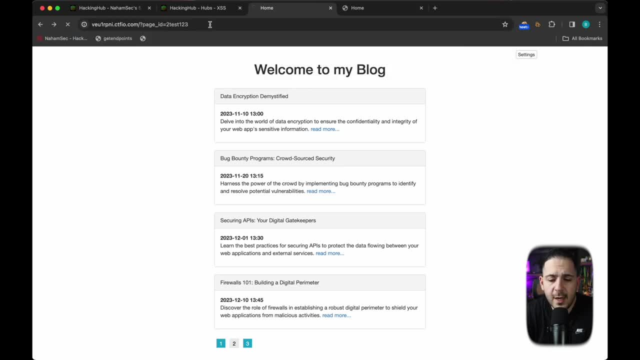 to put in a test123 for whatever parameter you want to test for, and we're going to send this exact request and see if test123 actually reflects or gets shown anywhere on the page. and as we do a command F and do a test123 search, nothing shows up. the next thing you want to do is you want to either: 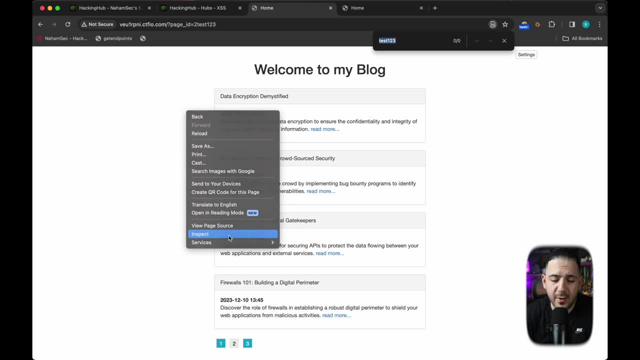 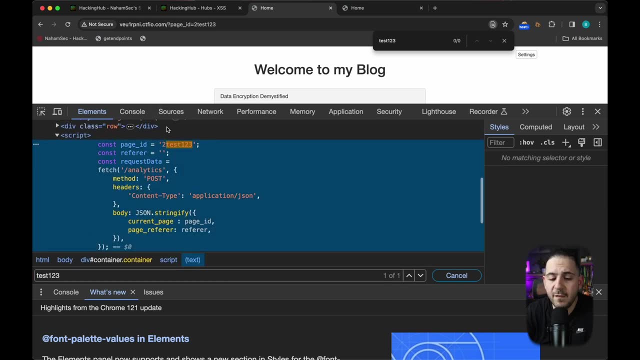 do a page source. honestly, it's better if you do inspect to get more data because of the Dom in there. so when I open up inspect and I'm going to look for the same exact thing, which is test123, and we can see that it's being reflected within the Dom, within the script tag. so the first thing you 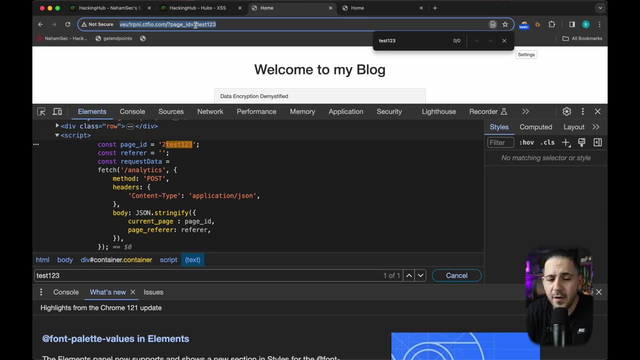 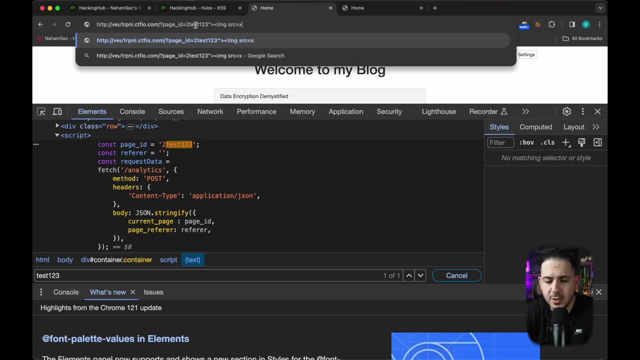 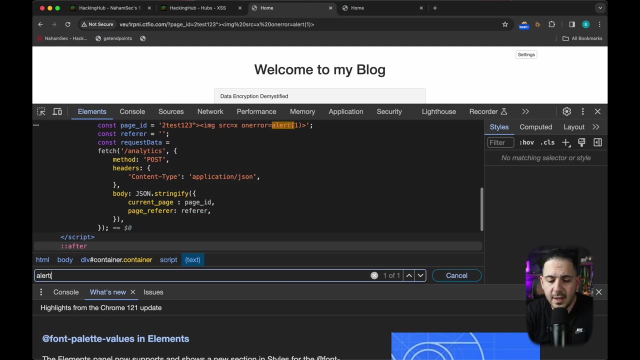 want to do is- and this is the reason why I tell everybody to stay away from just copy pasting payloads- is because if you copy paste a payload, for example, let's do something like an image. if we send this, even though it is a valid access payload, it is not going to pop up because we are 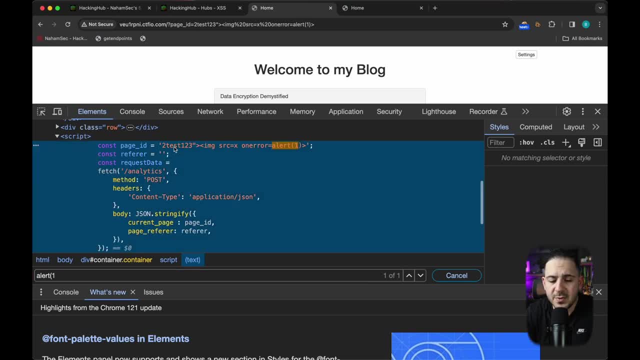 in a context of a script, you always want to see where your test reflects and kind of play around with it and get out of that context before you include some JavaScript. in this case we're on a script tag. sometimes you're going to be in a text format, so it's a text area. sometimes it might be. 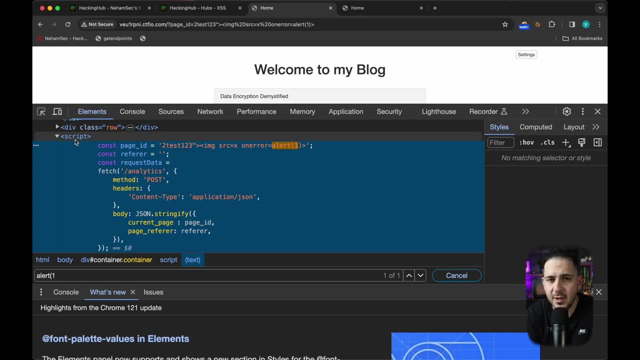 in a title, all of those, it's the same. if you give it a valid HTML payload or an XSS payload, that's not going to fire. so what we're going to do here is we're going to see that we're in a script tag. we need to close the script tag and in html, all you have to do is do: 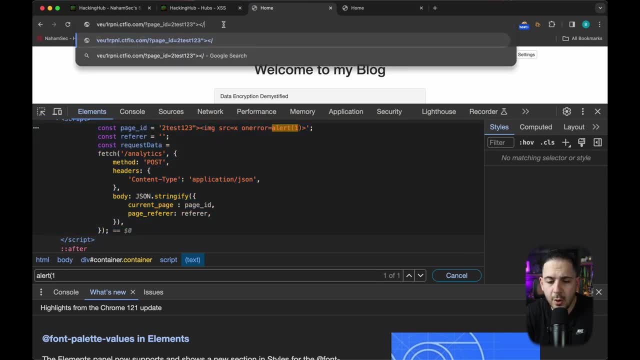 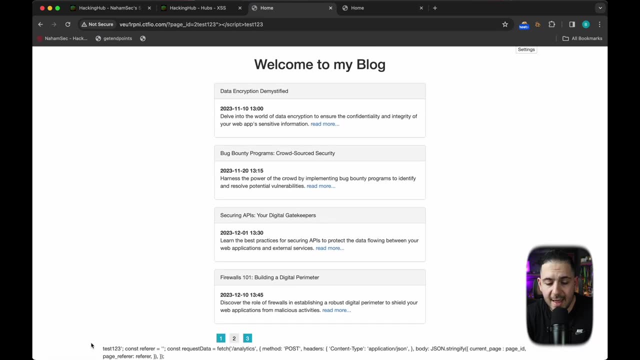 the same tag and put a closing bracket against it. so we're going to do a script and then we're going to test, put out test one, two, three and see if it changed anything on the page. it looks like now we have broken out of the html and at the bottom of the page we actually have some stuff. 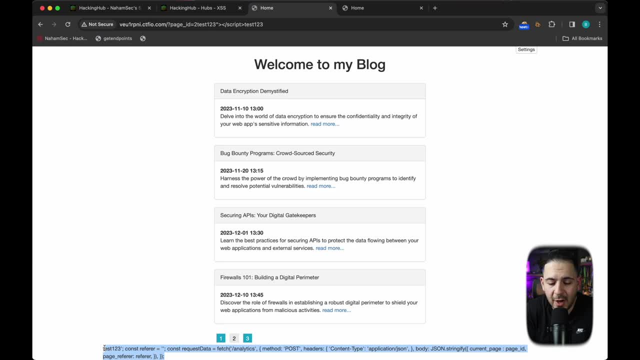 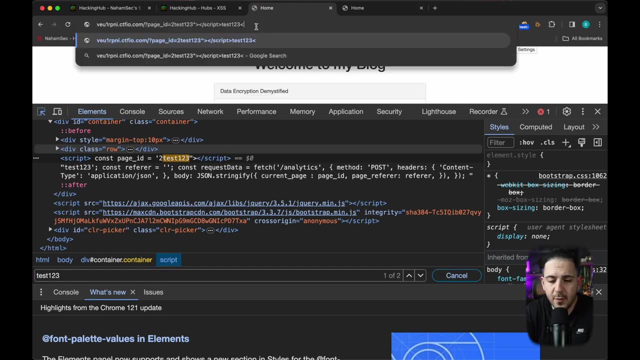 that has leaked because we've closed out the script tag and the browser doesn't know what to do with the leftovers. so what we're going to do here is we're going to go back to our test one, two, three here and we're just going to add whatever payload we want, whether it's image source we want. 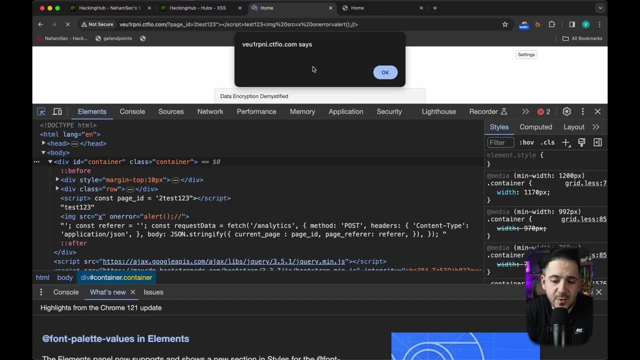 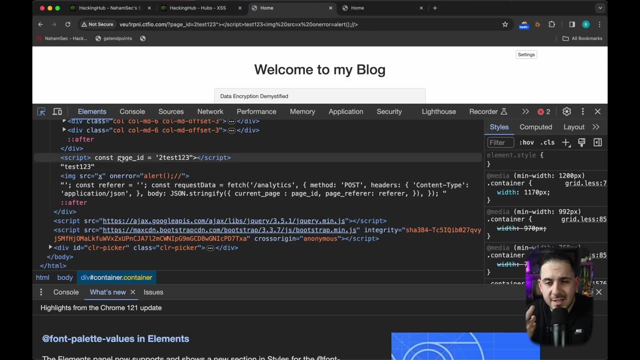 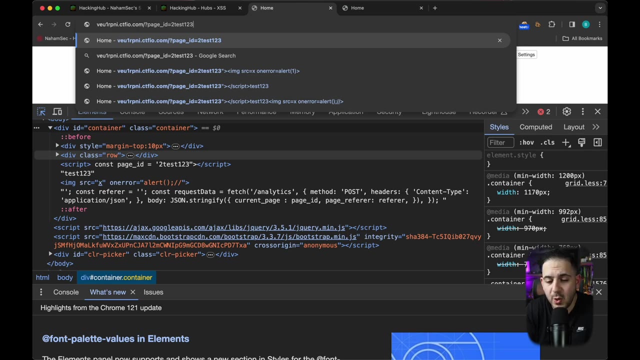 to do a xss and so on and, as you can see right there, it pops up with our alert, and the only reason why this works is because we looked into the dom and we saw that we are in a script tag and we want to close that out. you also have the capability of not having to actually close. 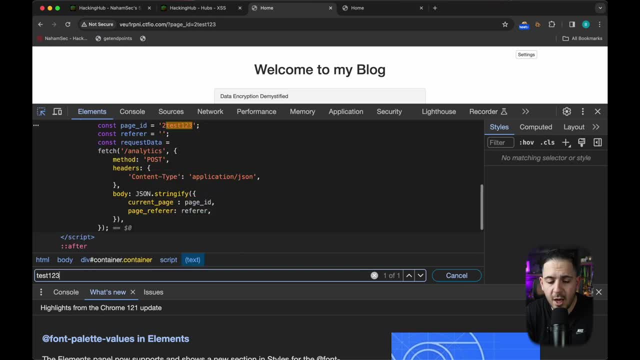 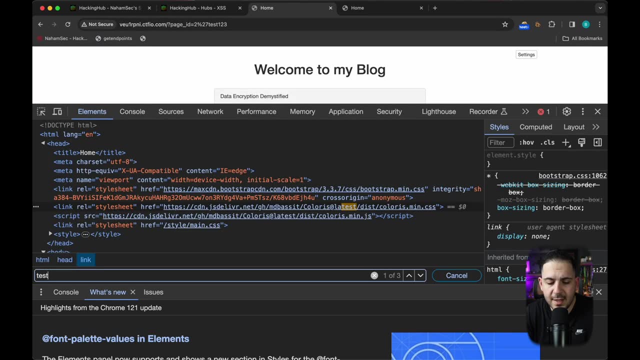 the script tags. if we look at test one, two, three again, sometimes you may not be able to close the script tag and all you have to do is just close that parameter and you're going to be able to say, hey, i want to say two. and then we look right here we can see that this two right here is having. 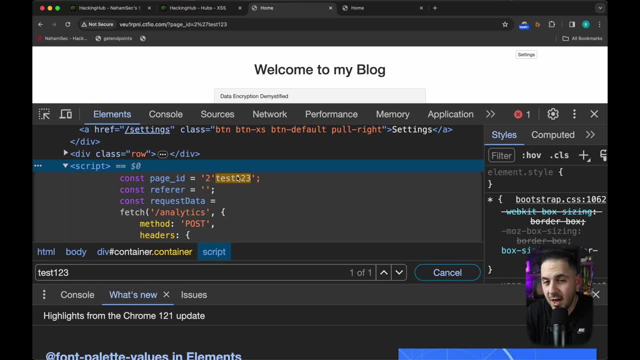 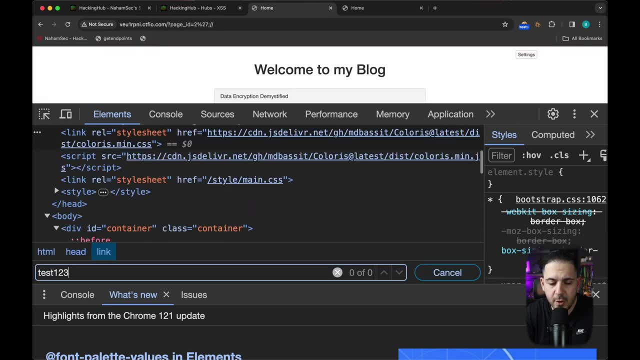 an extra apostrophe and then the rest of it, and this is not a valid javascript, but what we want to do is, now that we have closed it out, we can comment the rest of it out, so, and if we look for it again, we can stop. let's do test one, two, three at the end of this, just so we're we know where to. 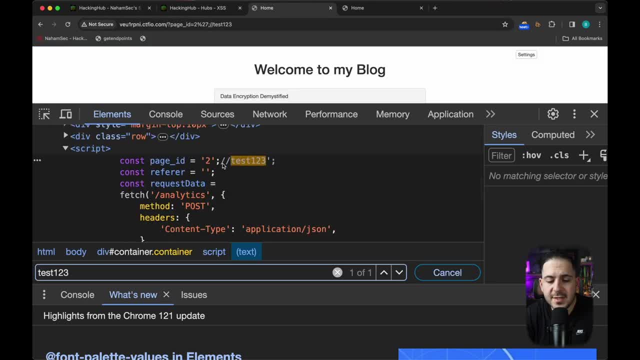 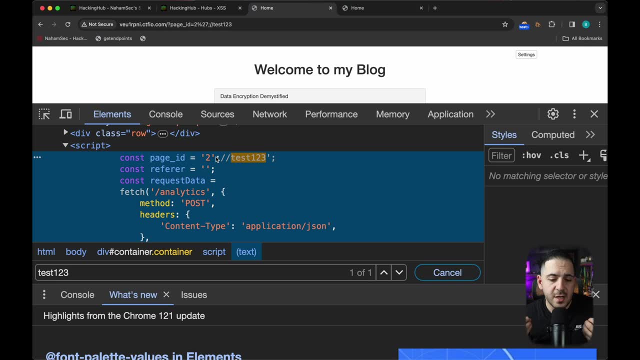 look for it. if we look for test one, two, three, we can see that we have valid javascript. we've closed the pass parameter, but now we want to introduce a javascript alert into this, and let me type this in really quickly right here. what we're going to do is: 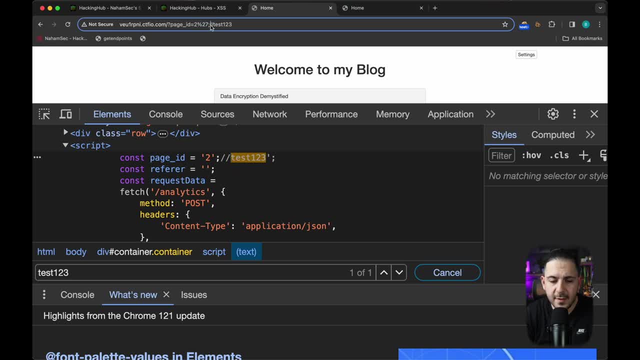 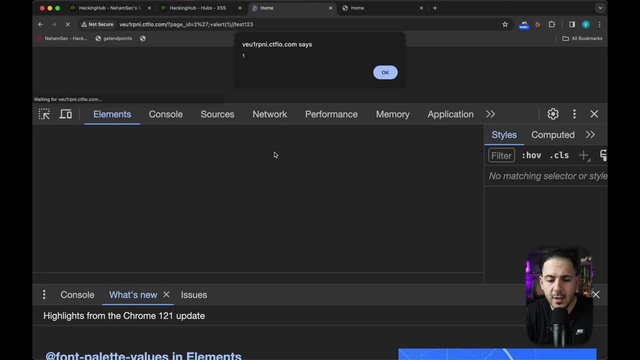 since we've already closed the apostrophe right here. that's what we've inserted. then we have our semicolon. that's what it is. then we're going to give it a plus and then whatever function we want to call- in this case we want to call alert one. by doing that, it works. the alert one works out now. 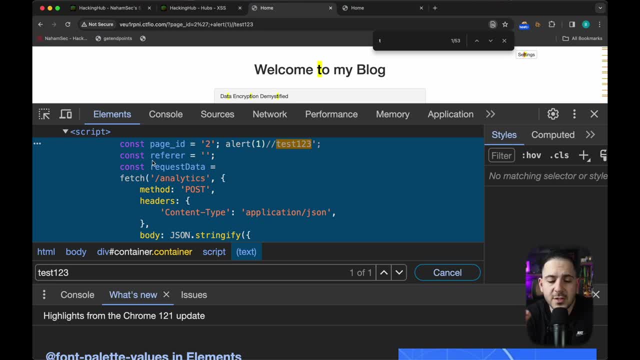 what we want to do is we want to also take a look at all the different variables that may be called referrer, which has an empty value, and you can see page id is pretty much what we have put up here. that is reflecting in the source and a lot of times what i want to do when i do a test and i 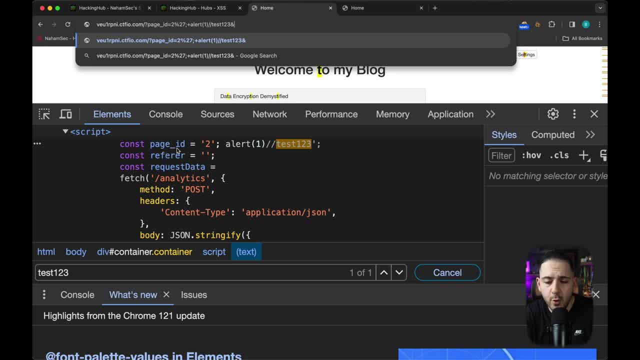 see something empty like that right under another variable or parameter that was used. i always want to just check it out. i'm going to put in referrer and then do a. maybe we can do just a five-week program, one, two, three for this one. let's try it one more time. we can ignore the alert. we can. 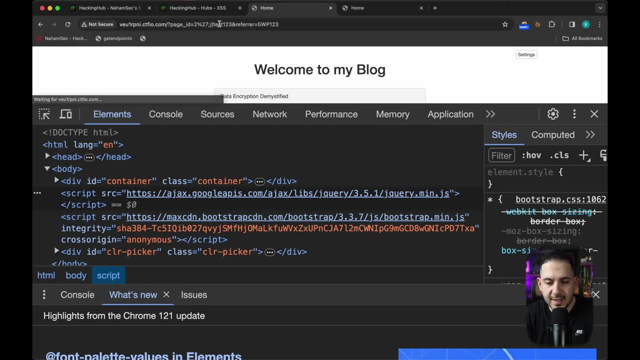 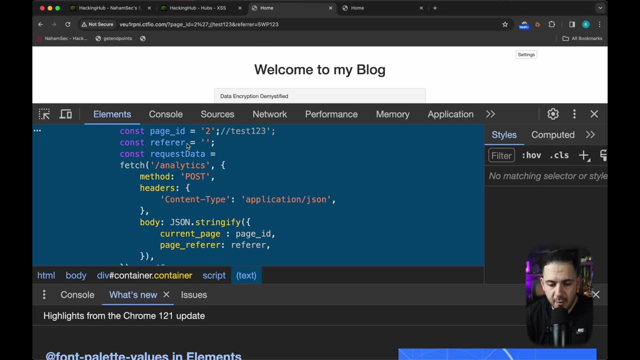 actually remove it so it's not annoying us anymore. we're going to send that out and then we're going to do wp one, two, three. nothing comes up. so you can see, in this one maybe referrer doesn't work. actually looks like we have a typo, so let's do a one r. it's really important to make sure you. 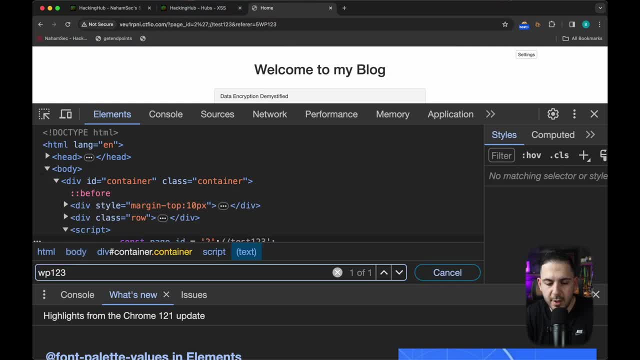 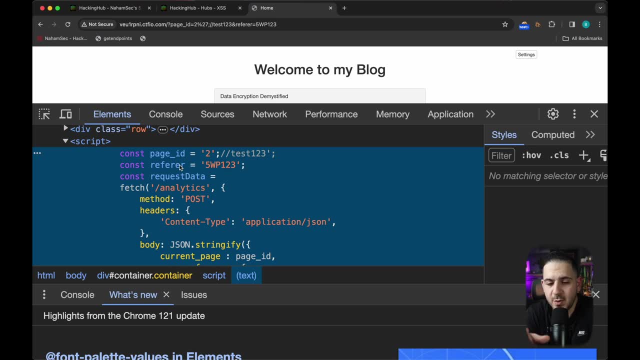 actually do this properly. we're going to do one, two, three test. one, two, three. there we go. now we can see right here underneath the referrer: even though we didn't see it on the page, it was not mentioned to us, we can see it exists under our javascript. right here it says referrer we put 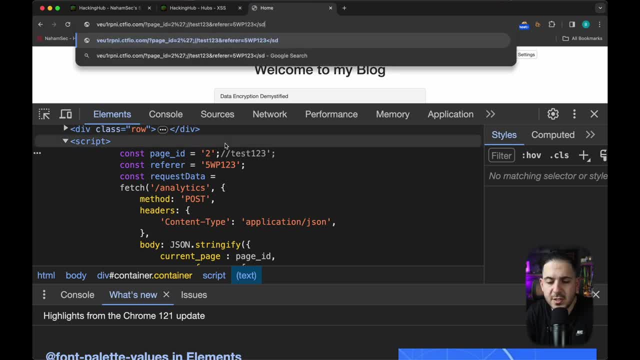 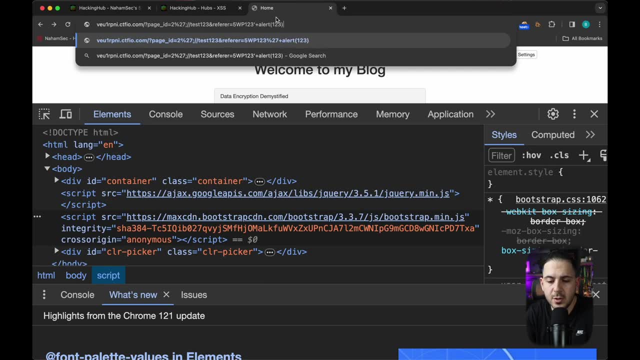 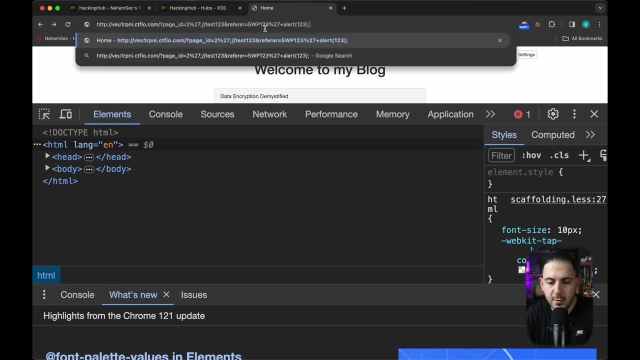 it up. it reflects the concept, is the same thing. we can just do a script or we can just do: uh, close that one out, and say: close that one out, and then do an alert- one, two, three- and then seeing if that works as well, let's see what didn't work. i forgot a semicolon, so let me just put that in there and 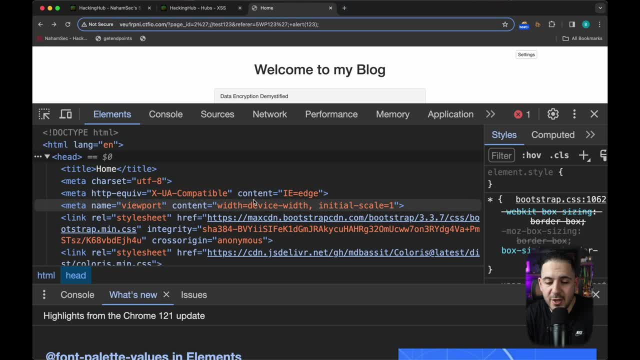 let's see what calls it this time. it's also really important to actually comment out all of the rest of this javascript that is not going to be valid because the browser is going to look at it and go: but what am i supposed to do? i'm going to do this, and then i'm going to do this, and then i'm going. 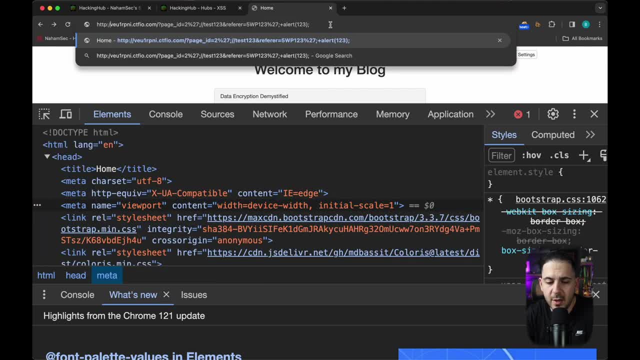 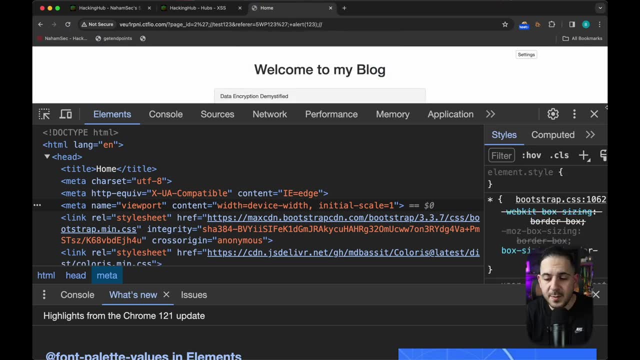 to do with the rest of this. so what we're going to do is we're going to just comment that out as well, and now we can see alert one, two, three work. so that's a really good place to start with cross-site scripting. you always want to just do your first value, first see what context you're in. 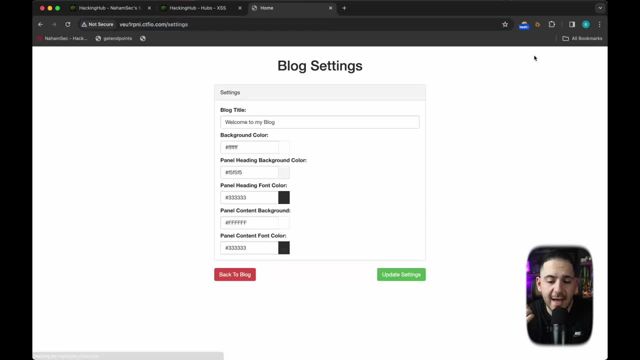 and then go from there. the second thing is, you also want to look at all the other fields that are presented to you within a web page. so, for example, one of my favorite things to look at a lot of times is customization, and a lot of times people miss this because they're not really 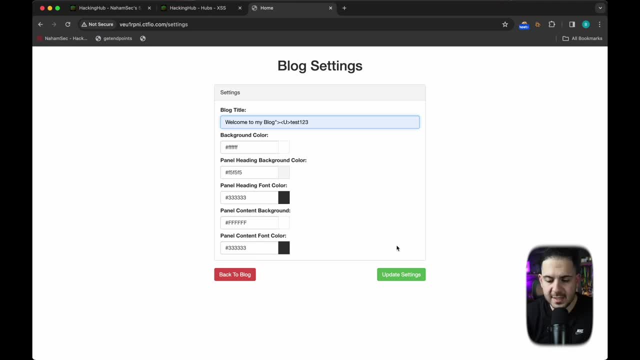 actually looking at it properly. so what we're going to do in this case is we're going to send the update settings. we're going to do the same thing. we're going to say: i'm just going to assume we're in some quotation, close the html tag and start our underline and update settings. it's going to. 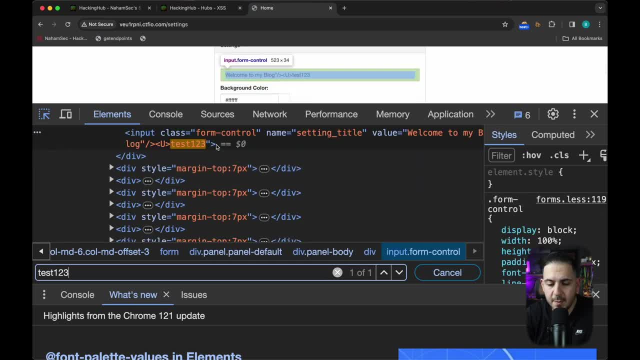 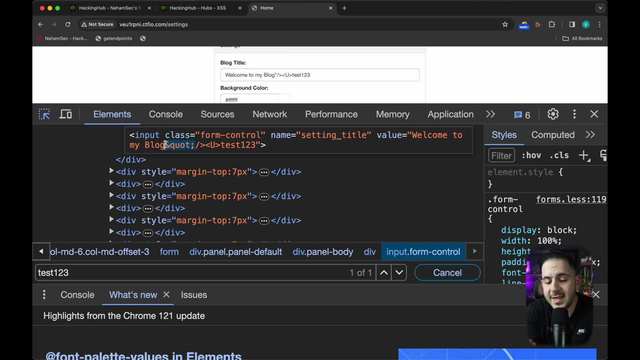 come back and obviously nothing works. and we're going to look this up. and if we click right here and do edit html, we can see that our quote right here was properly sanitized, so it doesn't let us actually do xss, then this may not be vulnerable. and right here, 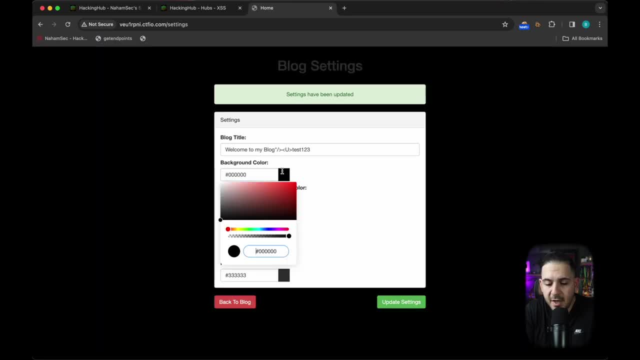 if we try to do some additional values and save it, it doesn't work. it's not taking that because there's some sort of a test. but here's where it gets interesting: just because on your browser itself you are not allowed to enter some sort of a value, it doesn't mean that it's not vulnerable. 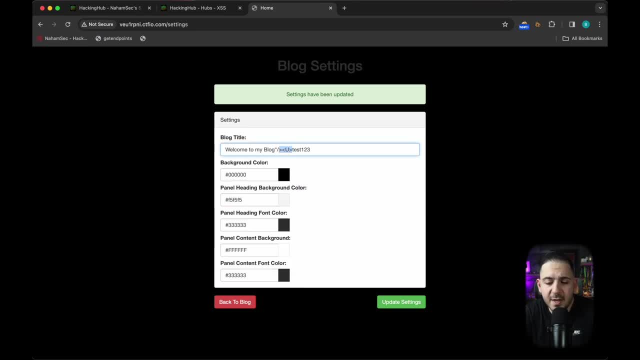 a lot of times what i see is, if i put even an html code right here at the bottom of the box, it says hey, no special characters are allowed. a lot of times people give up right there. and what i? what i recommend a lot of times is to go in here and actually remove it. 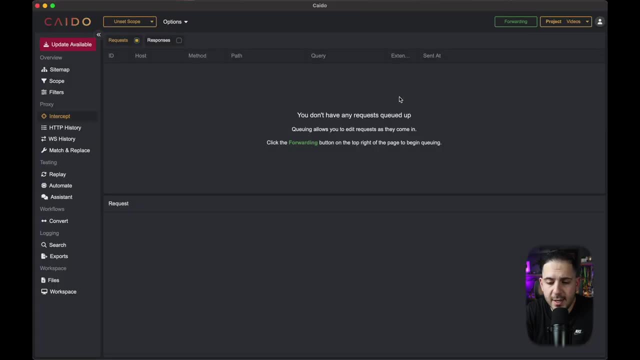 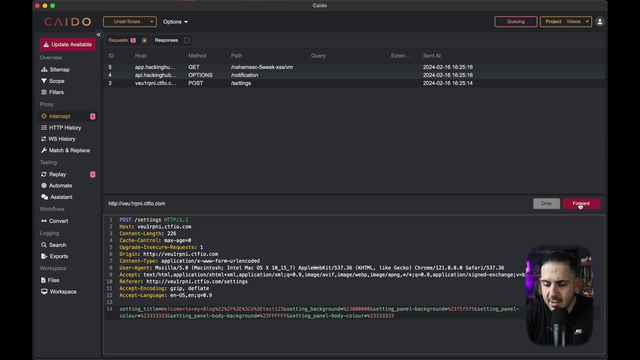 and put it in the post request. so what i'm going to do here, i'm going to go back to kaido. i'm going to start doing our queuing, i'm going to send this request and we can see sending a request to settings. i'm going to send it to my repeater and we're going to stop queuing this. go to replay. 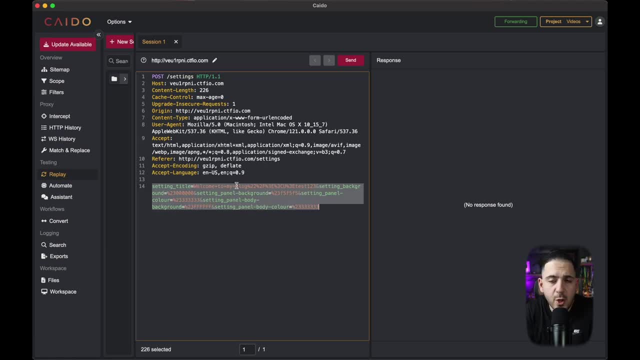 and right here we're going to see what we have. so for this first one, we know we can put special characters in, but it's not vulnerable. but what's really cool is that there's styling in here that we can actually mess with. and if you're not familiar with css, css usually starts- 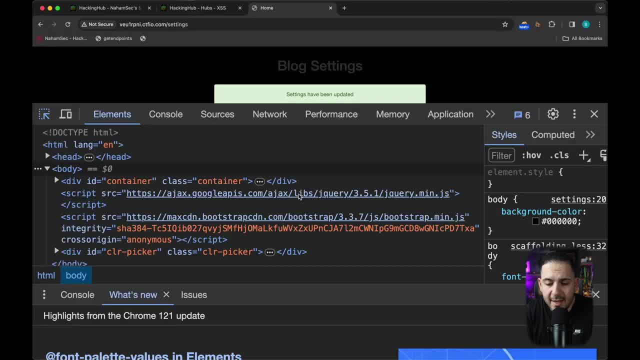 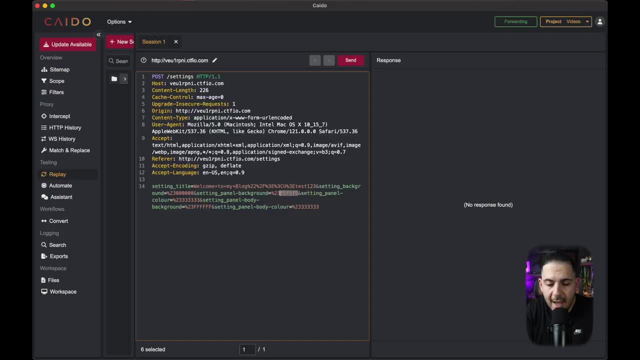 with a style. so if i actually copy this and go back in here and look for this code, you can see that it is being under a style tag and it's written right there. so what happens if we actually do this manually and put it in our request and say, hey, i want to close style and i want to add: 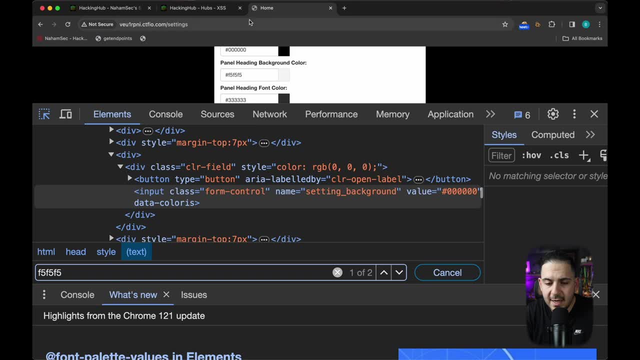 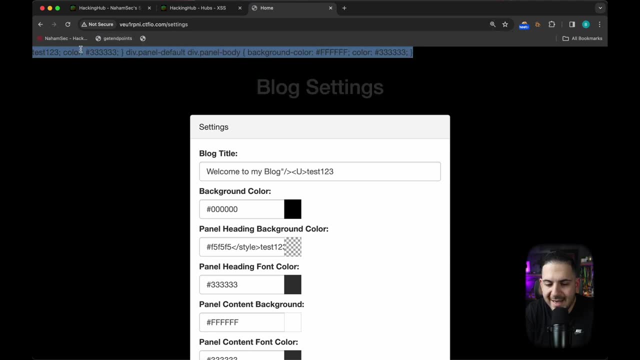 test one, two, three. let's send this and it will save. i'm going to go back to this page and reload it and at the top right here you can see that there is some text that's hidden. it's kind of leaking the remainder of the javascript, starting with test one, two, three, because we told it to. 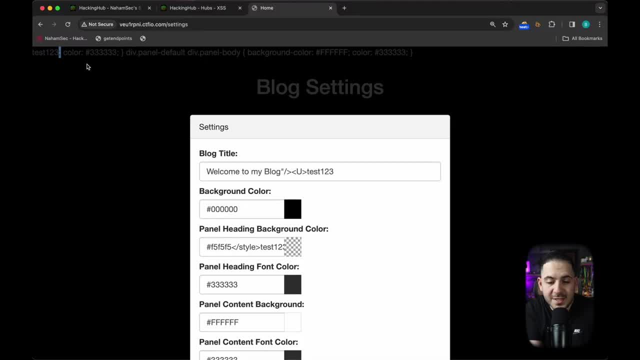 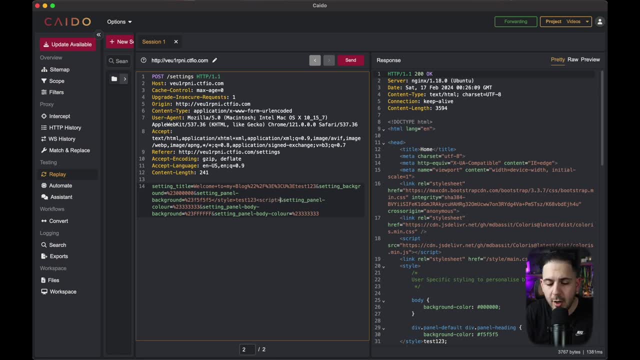 close the style and then add a test- one, two, three- that is vulnerable, so it's leaking everything. so what you want to do in this case is: this is why i say context is very, very important. what you want to do here is you want to insert your script alert, whatever you want to use, whatever payload you want. 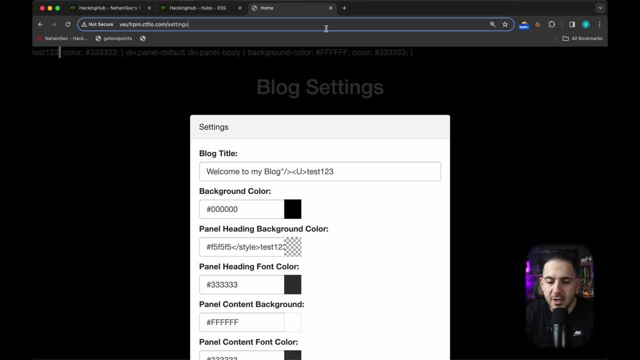 to use. you can put it in there and, as we refresh, i'm going to guarantee you that this is going to work. there we go. this one worked, so there it is. there's different ways you can look for crosshair. there's not always just based on the input that you can see and just because you see an error.